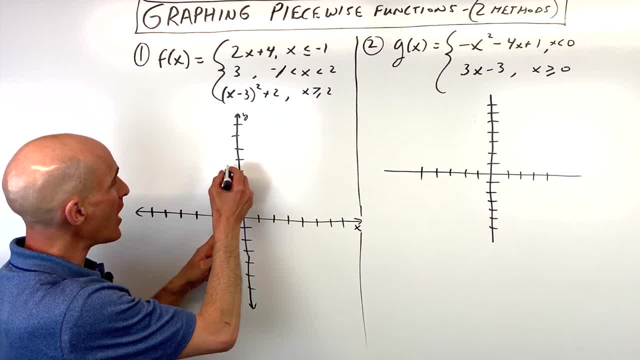 only when x is less than or equal to negative 1.. So what you can do, if you want, is go over here to where x is negative 1. I'm just going to draw like a dashed or dotted line. You can erase this later. 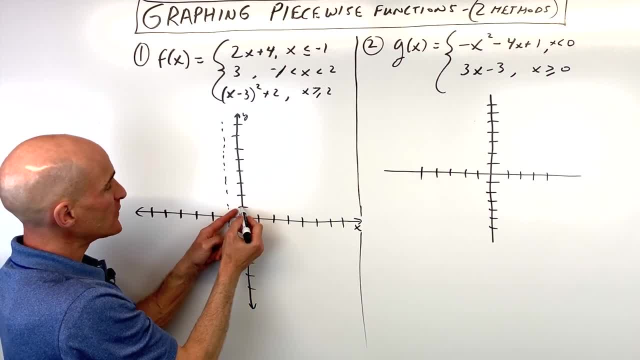 if you want, and what we're going to do is we're going to graph the line. y equals 2x plus 4.. It has a y-intercept of 4.. It has a slope of 2, which means we're going up 2 over 1,. okay, and you can. 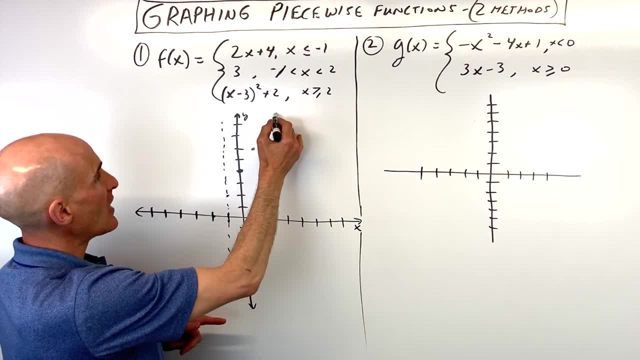 repeat that process, okay, and you can get your line like this, but we only want the part that's less than meaning to the left of the line. So we're going to graph: the line y equals 2x plus 4,. 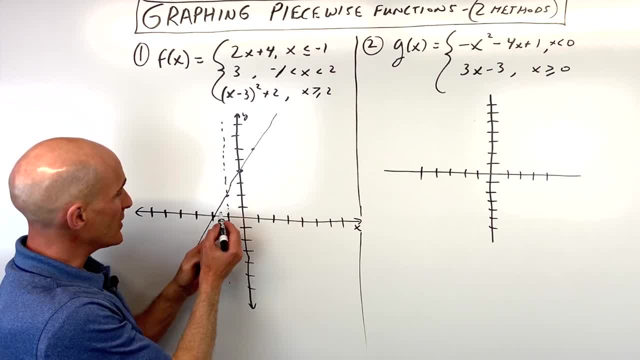 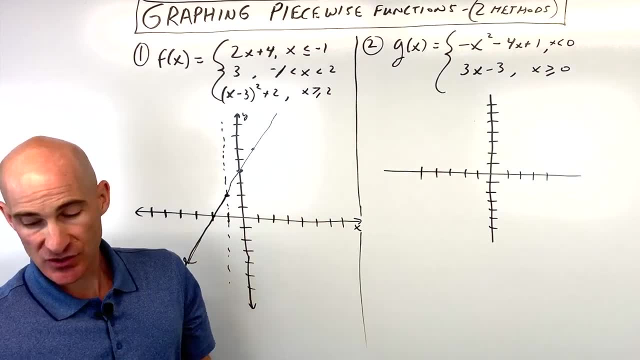 to the left of negative 1 or equal to negative 1.. So that means that this part here at negative 1 or to the left, meaning less than that's the part of the graph that we want. So the other part of the graph, I'm just going to go back and I'm going to erase, because we don't actually need that. 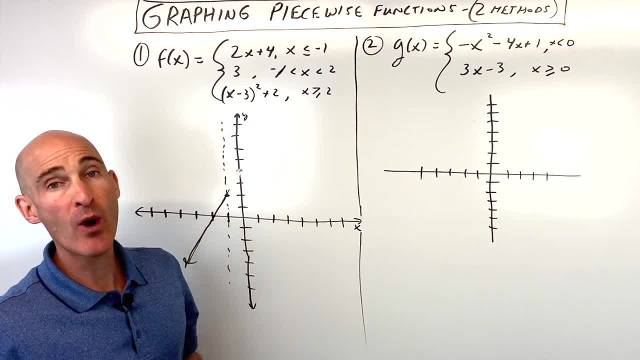 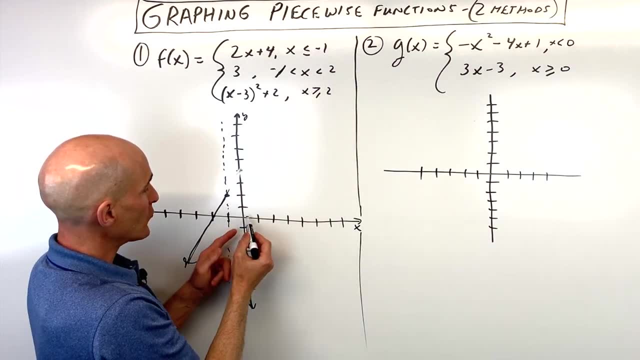 okay, So now the next part: y equals 3.. Now y equals lines. remember, these are horizontal lines. so I'm going to graph the line: y equals 3, but this is in between negative 1 and 2.. So if we go, 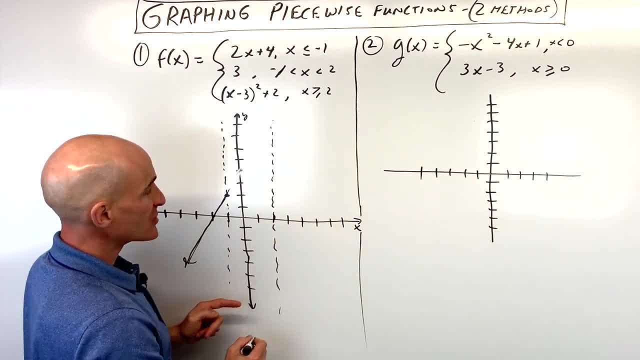 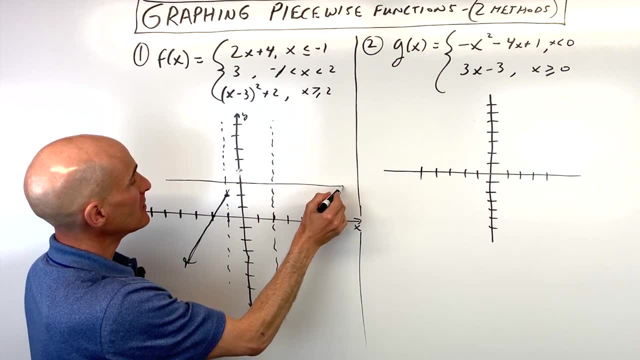 over here to x equals 2,. again, I'm just going to draw, like a light, a dashed or dotted line. We're going to be in between negative 1 and 2, and it's the line y equals 3.. So here's y equals 3, but we only want to be in between negative 1 and 2.. So, not including. 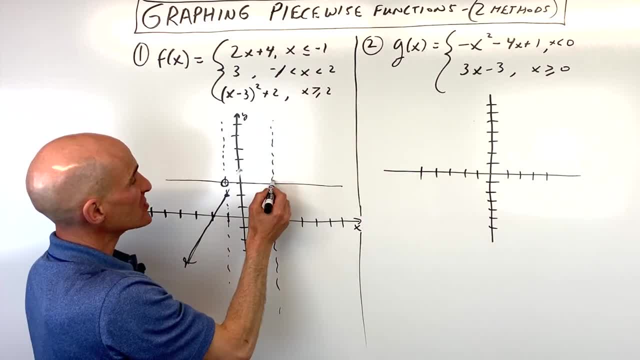 negative 1,. so this is going to be open, not including 2, but just less than 2.. So we're in between negative 1 and 2.. Notice, here this was less than or equal to negative 1.. That's why I 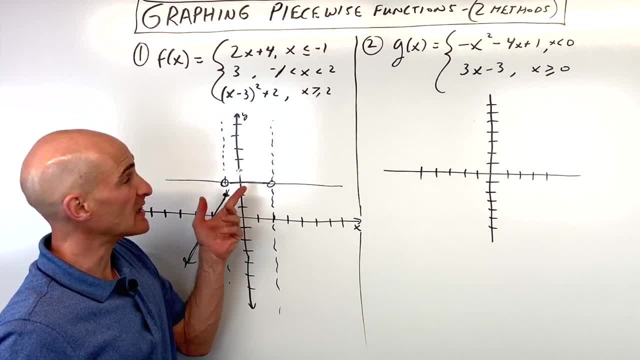 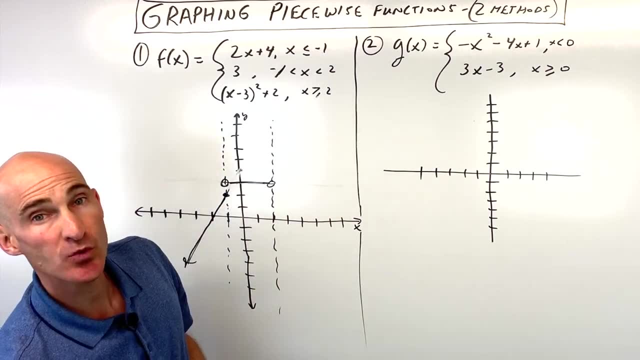 have this as a closed circle. It includes that point. This is open, meaning it doesn't include that point And the part of the graph that we don't need. now we're going to go back and we're going to erase. Okay, now, this is just one method. I'm going to show you another method. 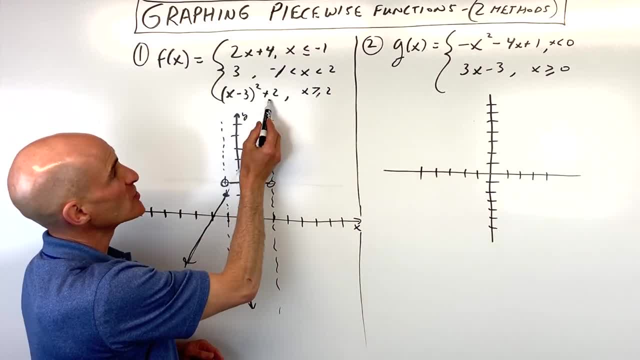 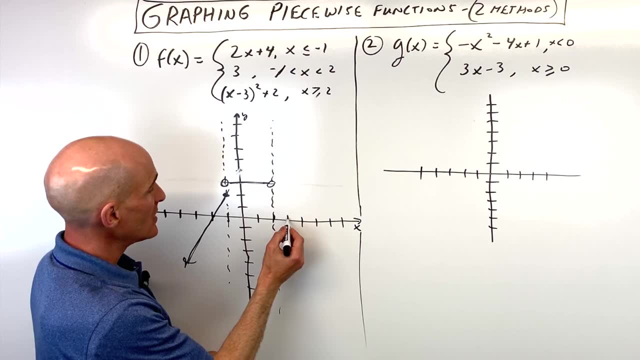 in number 2 here. The last part is: y equals x minus 3, squared plus 2.. We know this is a parabola. It's in vertex form. The vertex is positive 3, positive 2.. So I'm going to go over here to our 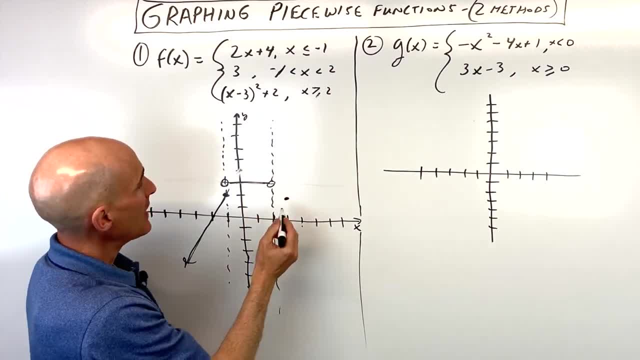 vertex. You can see the a value is 1.. It's opening up and you can see that this would be like if we plot some points. it's going to be like 1, 1,, 1, 1, and it's going to look like a parabola. 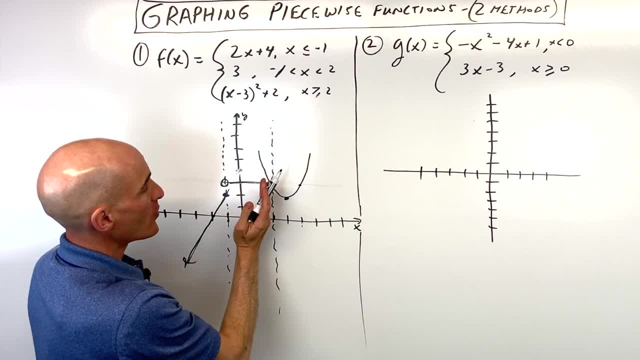 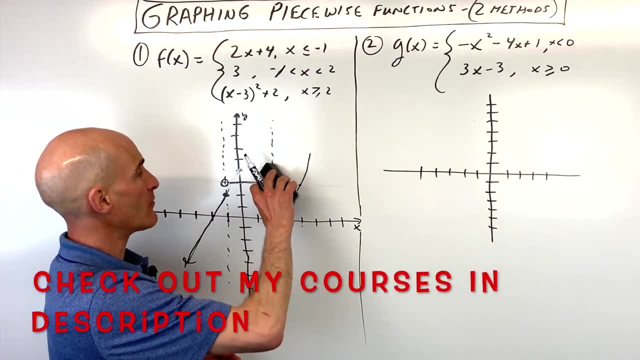 something like this: Okay, but we want the part where x is greater than meaning to the right of or equal to 2.. So this part here, that's to the left of 2, we don't actually need- I'm going to erase that portion there- and we just want the. 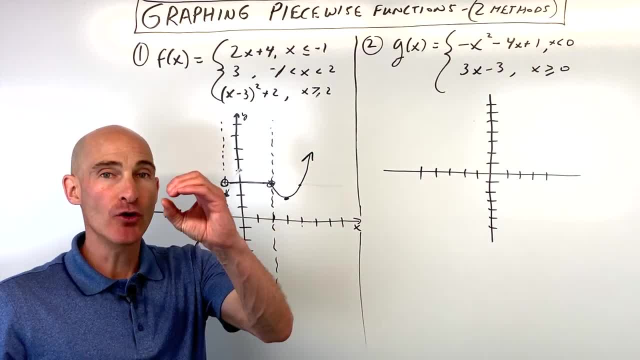 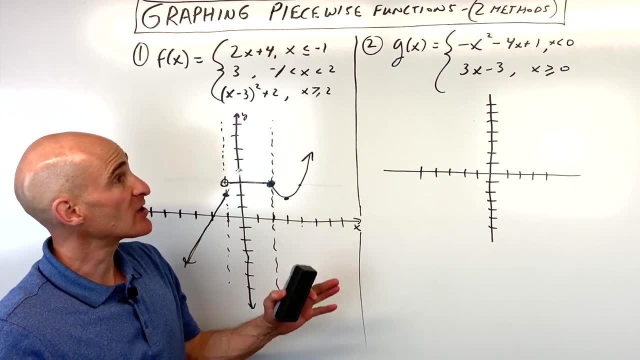 part greater than or equal to to the right. Now these ones happen to overlap the open part and the closed part, So that's going to end up being like a filled in circle. And that's it. Now you've got your piecewise function. Let's look at number 2. now I'm going to show you a different method. 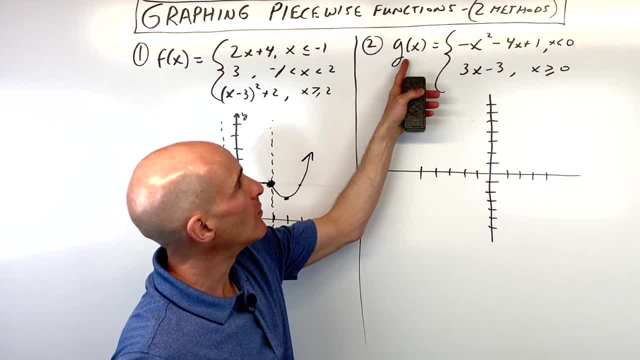 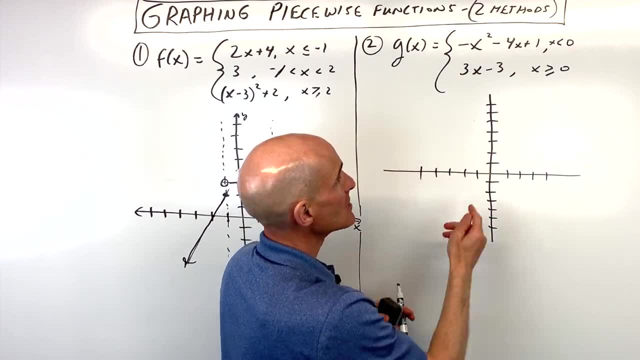 Some students like this method better, And what you're doing is you're graphing out these two functions. Now, here, the dividing line is: x is less than 0. So you're going to be able to divide it by 0, meaning, to the left of the y-axis, or x is greater than or equal to 0, so to the 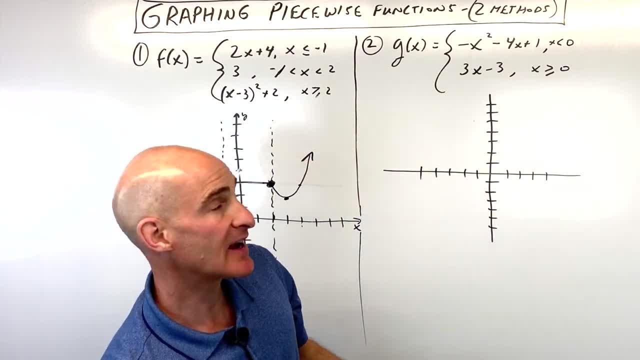 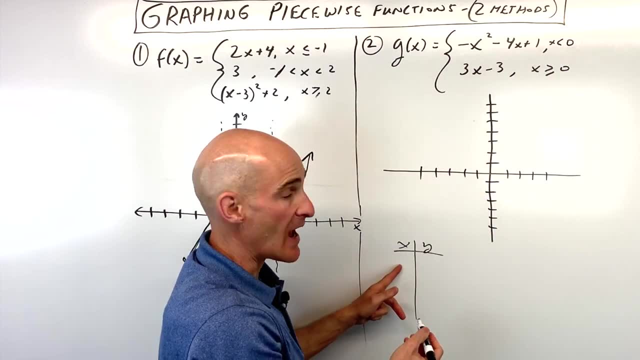 right of the y-axis. I'm not going to draw the lines here. We can just think of the y-axis as dividing it up into two parts. But what I'm going to do to show you here is I'm going to make a table and I'm going to pick values that are 0 or less. Now, 0, negative 1, negative 2, negative 3.. 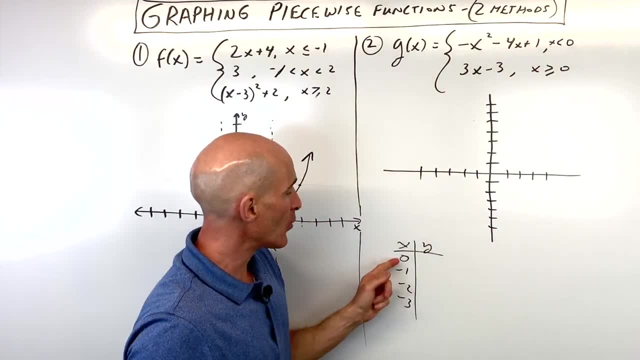 Now you might be saying: well, Mario, this is less than, but not equal to, 0.. But we're going to still put that point 0 in. I'm just going to draw it as an open circle on the graph, because it doesn't. 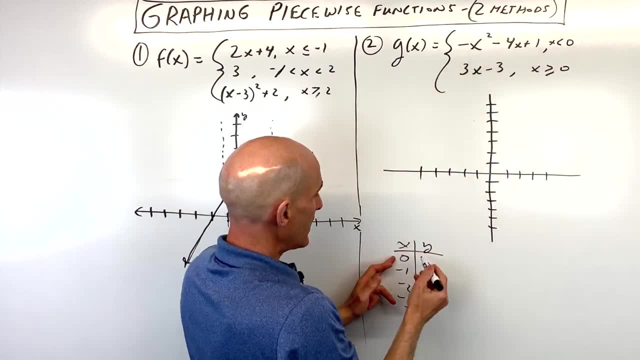 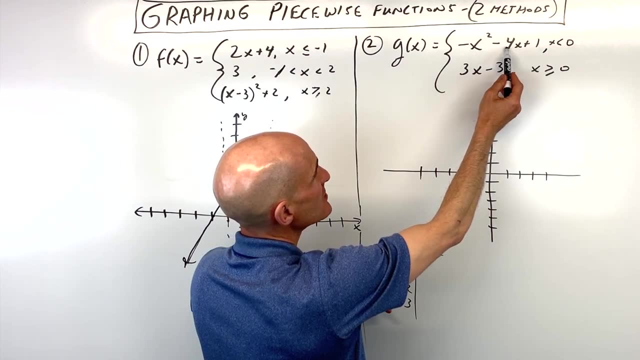 include 0.. So let's put 0 in, We get 1.. If I put negative 1 in, I get negative 1 squared is 1 times the negative is negative 1.. This will give you positive 4. So that's 3 plus 1 is 4.. Check. 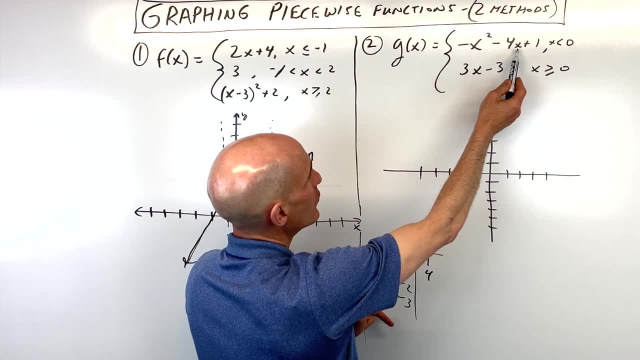 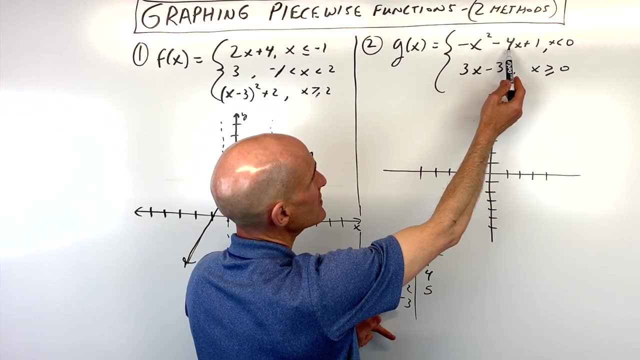 my math here. So this would be negative: 2 squared is 4.. That's negative 4 plus 8.. That's going to be 4 plus 1 is 5.. And negative 3 is going to give us negative 9 here plus 12. 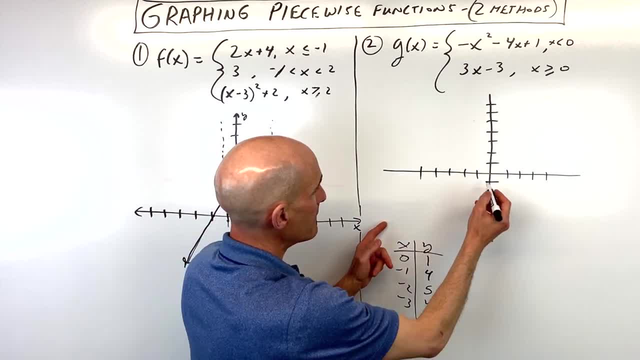 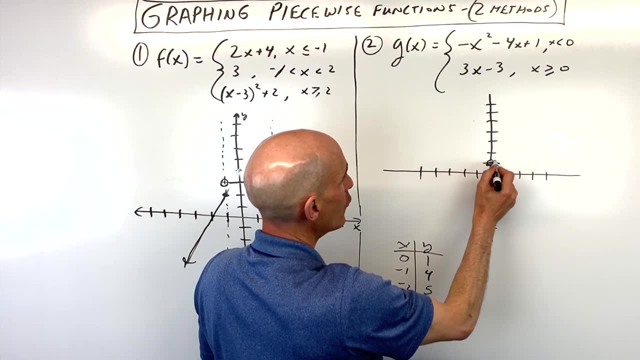 is 3 plus 1 is 4.. So if we graph these points, we get 0, 1.. And remember how that was: less than, but not equal to, 0. So this is actually going to be open. Open, not including that. 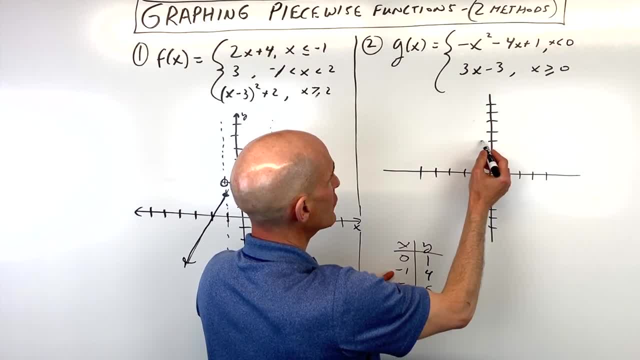 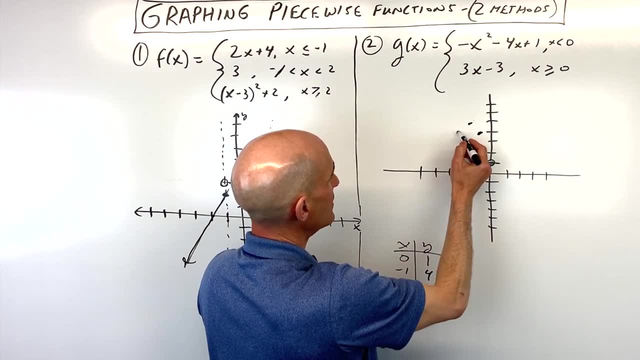 point. Negative 1 is going to be at 4.. 1,, 2,, 3, 4.. Negative 2, 5,, which is going to be right here. Negative 3, 4 is going to be right here. And remember how we said: we're less. 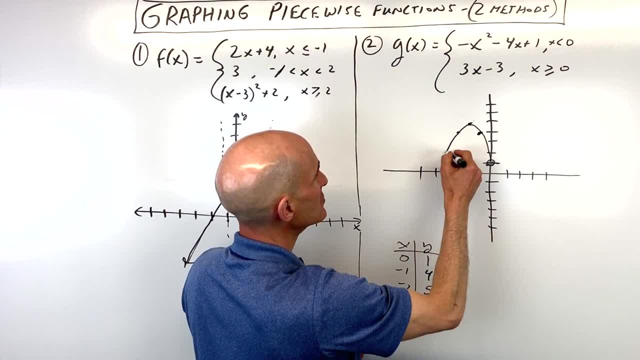 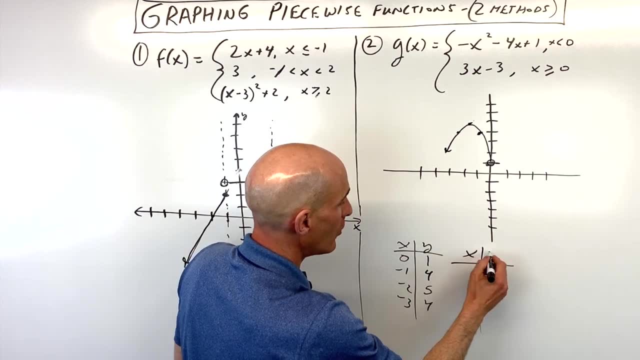 than, but not equal to, 0.. So it's just a part of the graph going to the left. of x equals 0.. Now for the second part: y equals 3x minus 3,. we're also going to make a table, but we're.